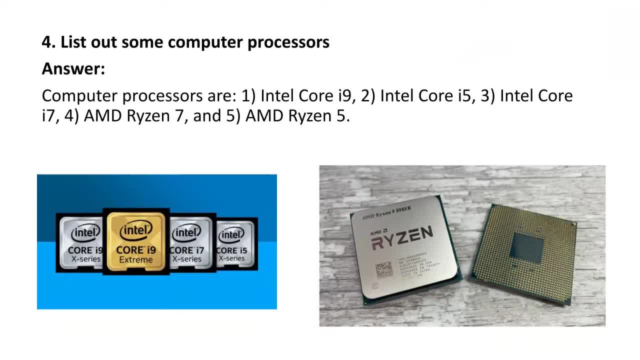 So the different computer processors are Intel Core 9, Intel Core 5, Intel Core i7, then AMD Ryzen 7, AMD Ryzen 5.. So these are nothing but different microprocessors with their generation. Next question: list out some popular operating system. 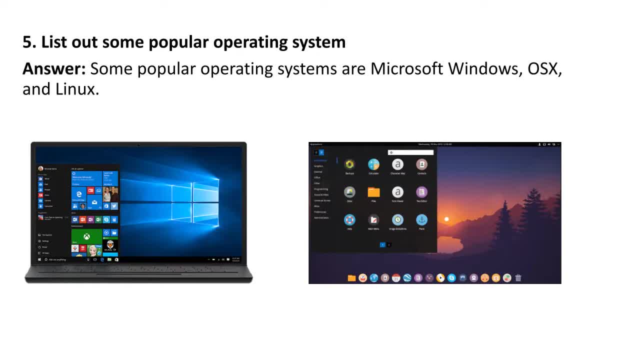 So the answer is: some popular operating system are Microsoft, Windows, OS X and Linux. So here in this image you can see the image at left hand side. it works on Windows operating system And the second one that is Linux operating system. 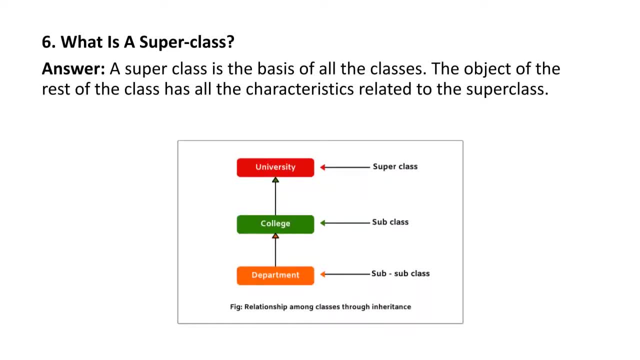 Next question: what is superclass? The answer is: a superclass is the basis of all classes. The object of rest of the class has all characteristics related to the superclass. So this can be understood with the help of this image. So here you can see, university is nothing but the superclass. 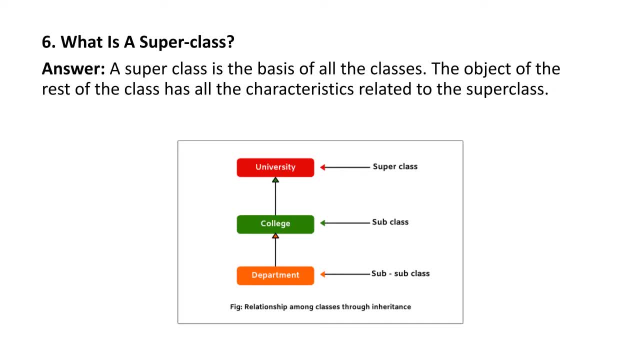 College is a subclass And the department that is sub-subclass, So the superclass is a basis of all classes. So here university is a base of college as well as department, And the object of rest of the class has all characteristics related to the superclass. 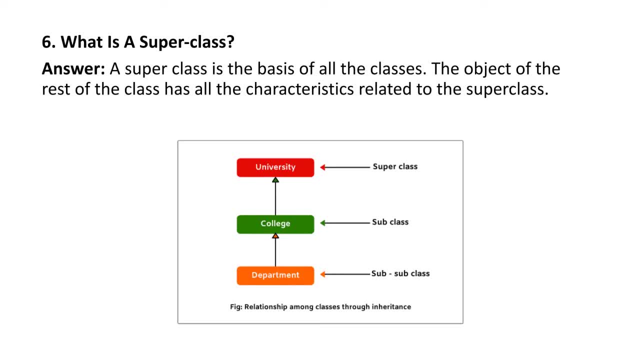 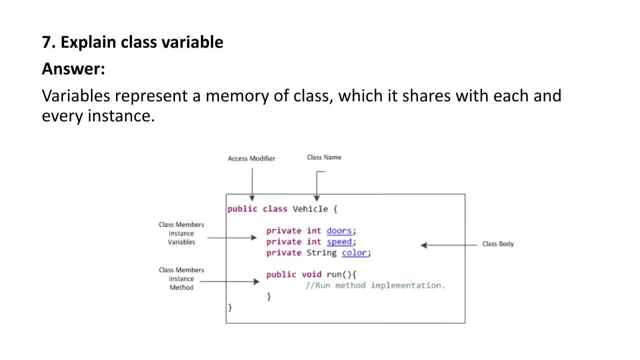 So the subclass college and sub-subclass, that is department. it has same characteristics to that of university. Next question: explain classes. What is class variable? So the answer is: variable: represent a memory of a class which it shares with each and every instance. 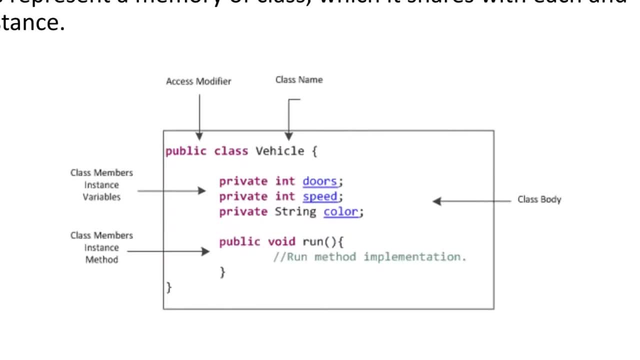 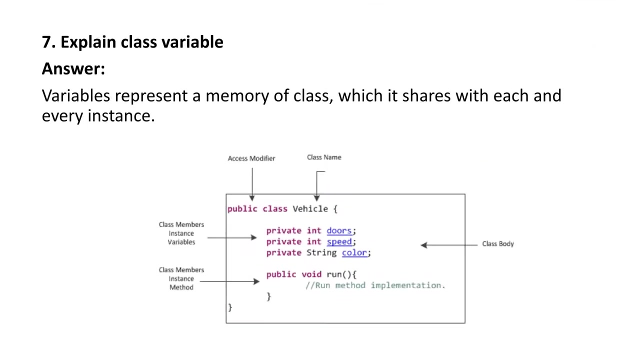 So here you can see, here I have taken vehicle as a class and public as a SS modifier And the instances of the vehicle, that is, door speed color. these are nothing but the characteristics of the vehicle. So the question was: what is class variable? 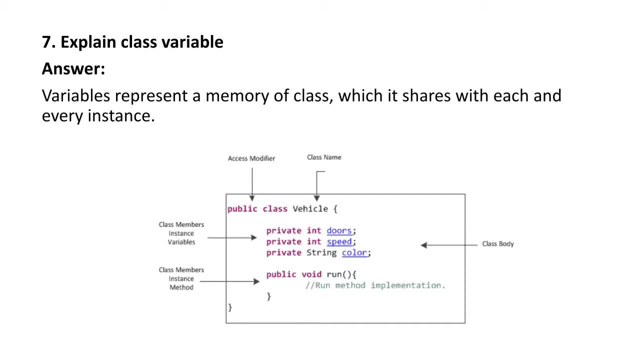 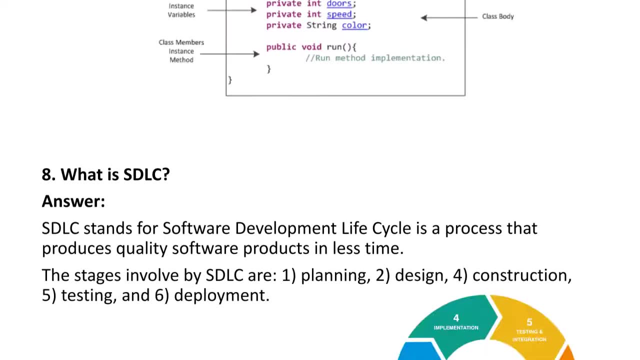 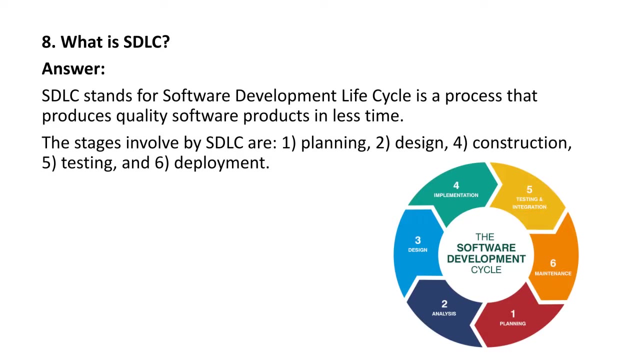 Variable represent a memory of a class which it shares with each and every instance. So this can be understood with the help of this image. Next question: what is SDLC? So the answer is: SDLC stands for software development. life cycle is a process that produce quality software products in less time. 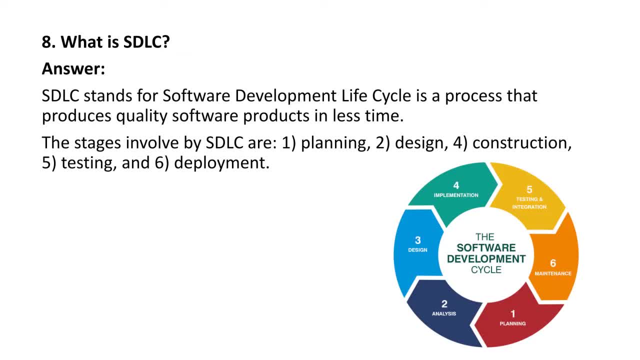 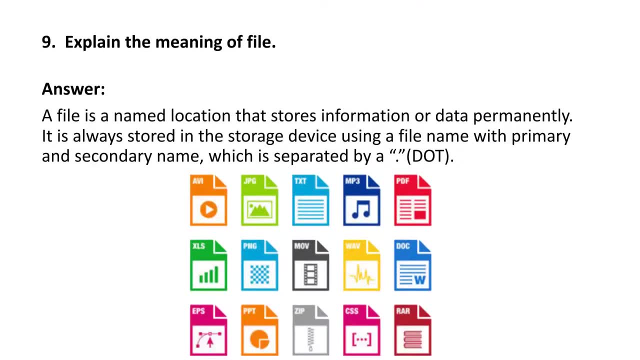 The stages involved in SDLC are planning, design, construction, testing and deployment. Next question: explain the meaning of a file. The answer is: a file is a named location that stores the information or data permanently. So basically, we are creating a file to store the information. 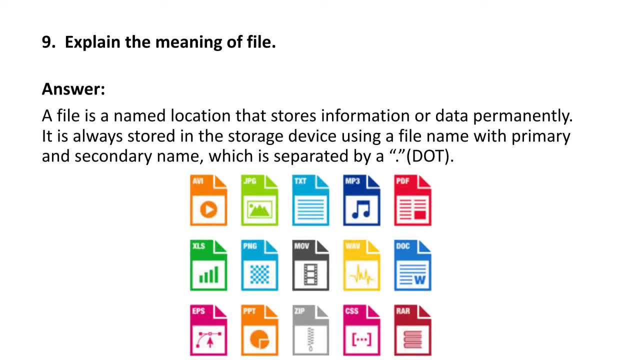 It always stored in the storage device using a file name with primary and secondary name which is separated by a dot. So you have to give a particular name to that file And that file has an extension which is separated by a dot. So here you can see different example of file. 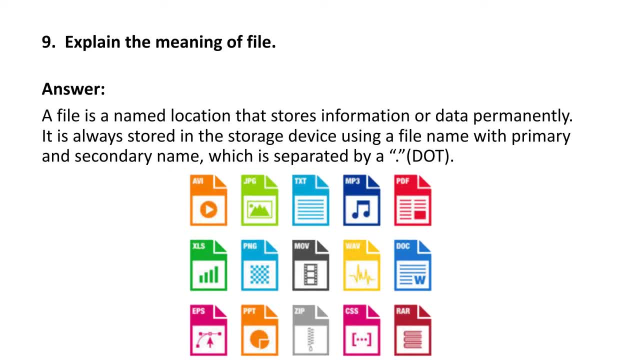 So AVI, that is a video file, Then JPG, it's an image file, TXT, it's a notepad file, MP3, again it's an audio file. PDF, XLS, that is Microsoft Excel file, Then DOC, PPT, ZIP, RAR. 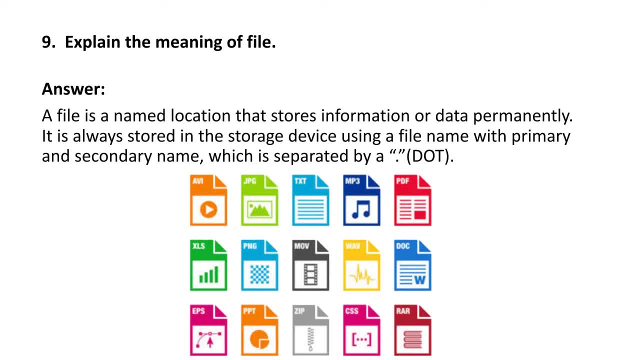 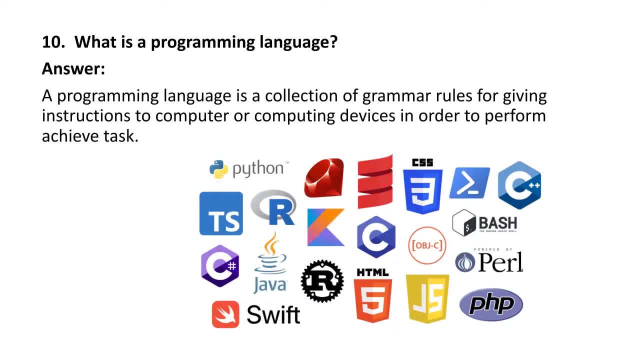 So these are nothing but different types of a file. Next question: what is programming language? The answer is: a programming language is a collection of grammar rules for giving instructions to the computer or computer devices in order to perform achieving task. So here the question is: what is programming language? 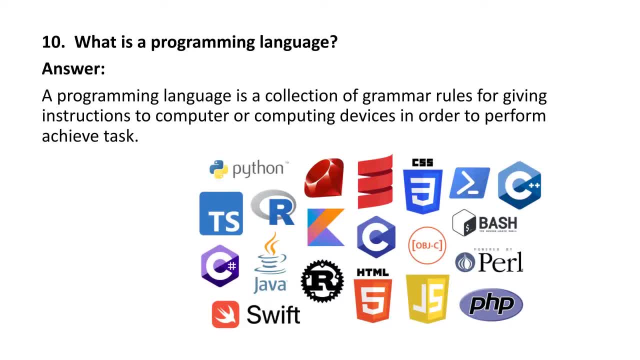 So programming language is a collection of grammar rules for giving instructions to the computer. So suppose you want to perform any task. for that purpose you have to write a program, And that program can be written with the help of a programming language. So with the help of this programming language, you can give instructions to the computer to perform a task. 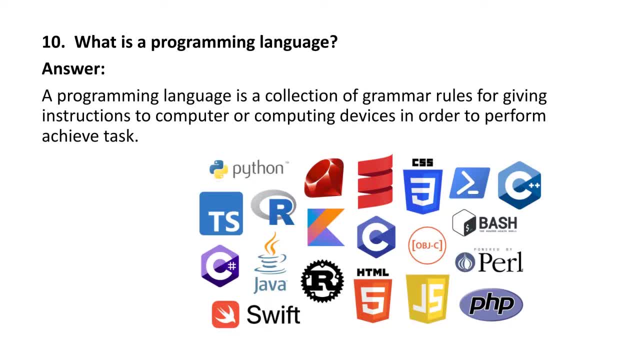 There are different types of programming language. Some of them I have listed here. So the very popular programming language that is Python, And the other language that is C, C++. This is the basic language. Some other languages like PHP, HTML, Java. 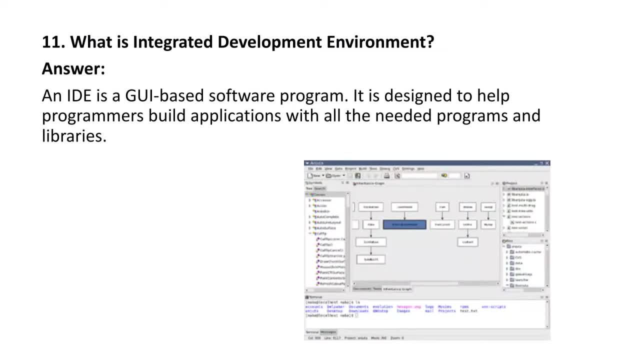 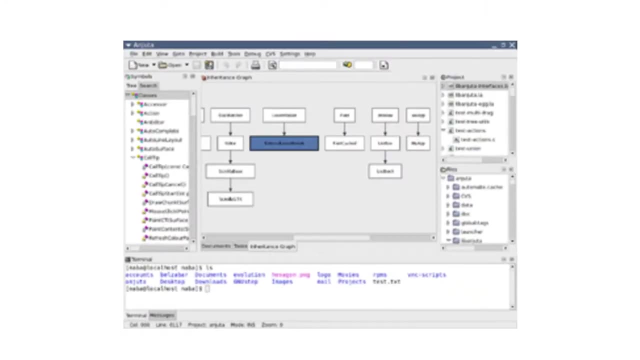 Next question: what is integrated development environment? The answer is an IDE, is a GUI based software program. It is designed to help programmer to build application with all the needed programs and libraries. So here you can see an example of GUI or you can say integrated development environment. 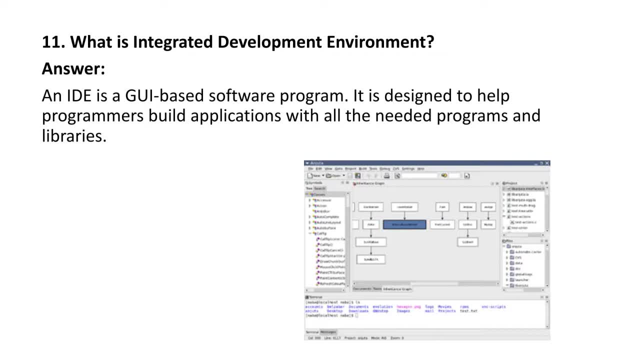 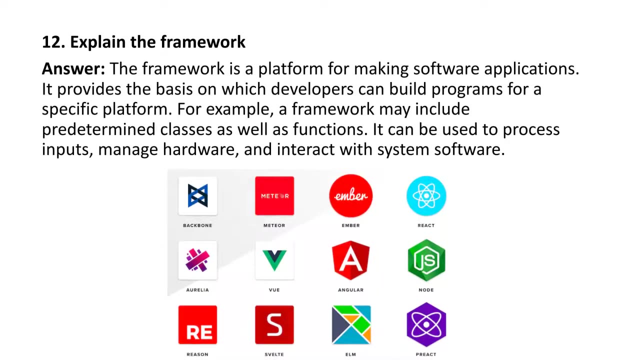 So it is basically meant for the programmer. With the help of this IDE, a programmer can build the application, because it will have some inbuilt functions and the libraries. Next question: explain the framework. The answer is: the framework is a platform for making software application. 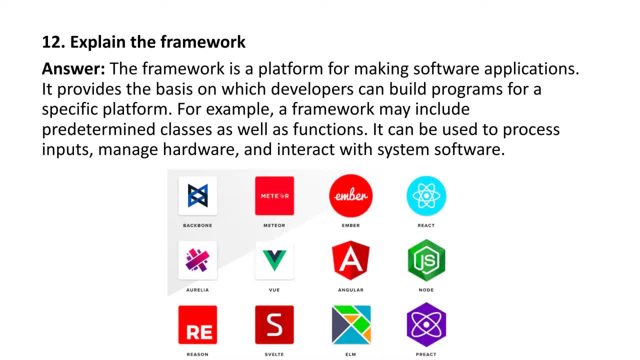 So, with the help of framework, a programmer can build a software application. It provides the basis on which developer can build the program for a specific platform. For example, a framework may include pre-determined classes as well as function. It can be used to process, input, manage hardware. 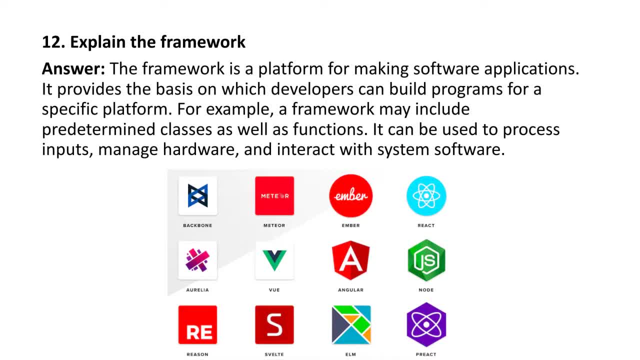 and interact with the system software. So basically a framework is used for making software application. It helps the programmer for building the software application. It will have some pre-determined classes as well as function. A programmer can use those classes and functions to build various application. 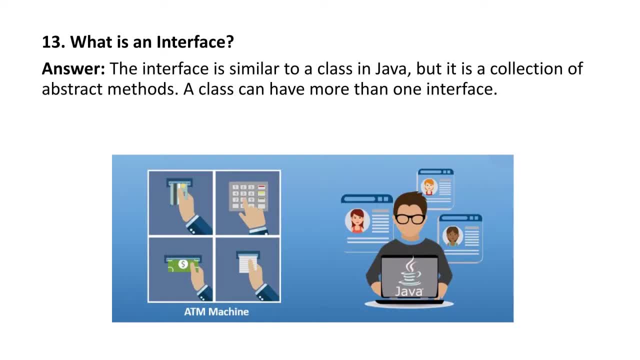 Next question: what is an interface? The answer is: the interface is similar to a class in Java, But it is a collection of abstract method. A class can have more than one interface, So this can be understood with the help of this image. 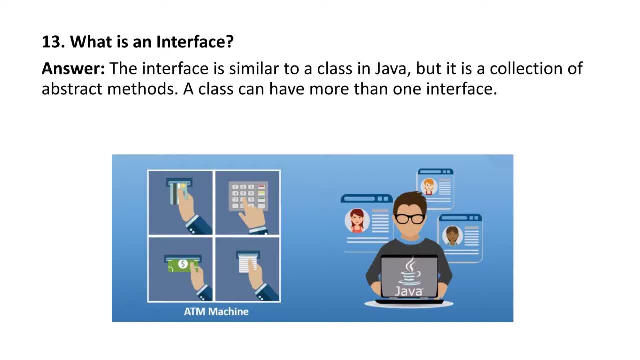 So whenever you visit the ATM machine you have to interact with that machine for withdrawal of money. So you will have one screen and there will be few options. So that screen is nothing but the interface. You have to click on a specific option to perform the task. 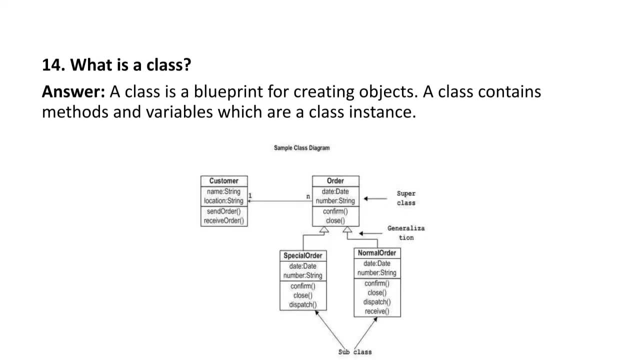 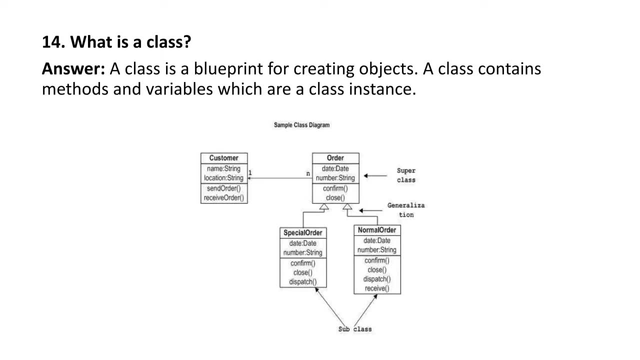 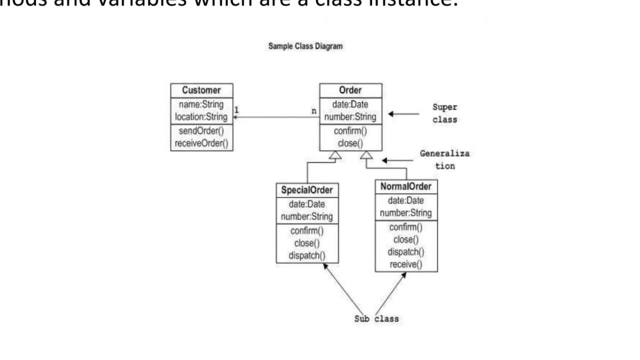 So that is nothing but the interface. Next question: what is class? The answer is: a class is a blueprint for creating the object. A class contains method and variable, which are a class instance. So here you can see the different classes. that is customer order. 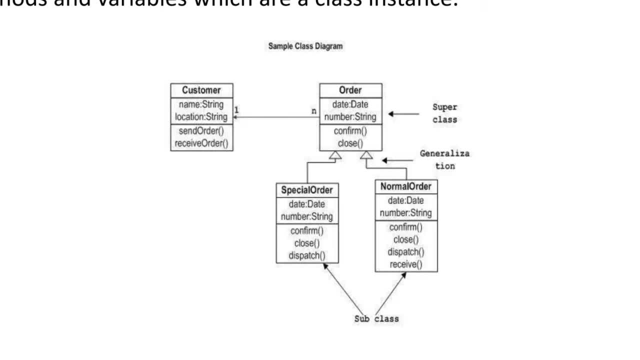 It will have some characteristics. that is nothing but the instance, That is the name of the customer, location of the customer For order. you can take the date of the order, the number, So this is nothing but the class. Next question: distinguish between abstract class and the interface. 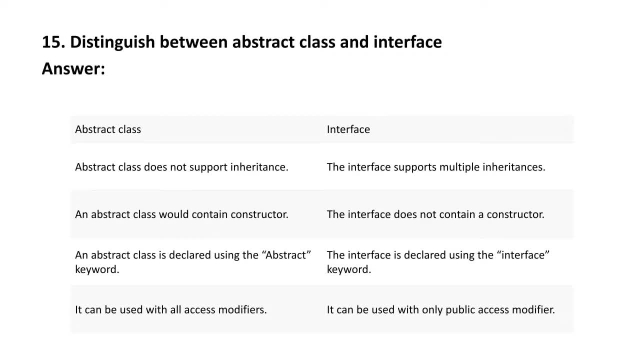 So the answer is: abstract class does not support inheritance. So inheritance is nothing but one of the concept in object oriented programming. So your abstract class does not support inheritance, Whereas the interface supports multiple inheritances. Then the next difference: an abstract class would contain constructor. 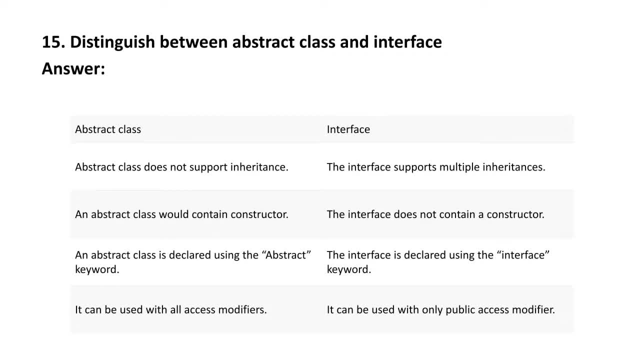 Whereas the interface does not contain the constructor. Next difference: an abstract class is declared using an abstract keyword. This is very important. So an abstract class is declared using an abstract keyword Whereas the interface is declared using interface keyword. Then the abstract class can be used with all access modifier. 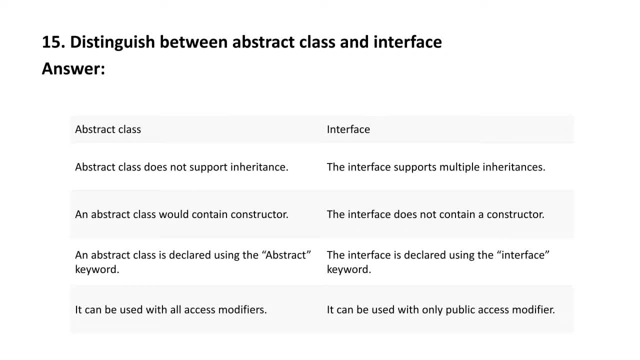 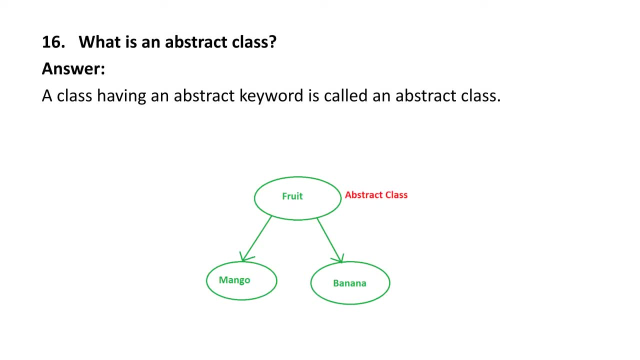 Whereas the interface can be used with only public access modifier. So this is the difference between abstract class and the interface. Next question: what is an abstract class? This is very basic question: What is an abstract class? So a class having an abstract keyword is called as an abstract class. 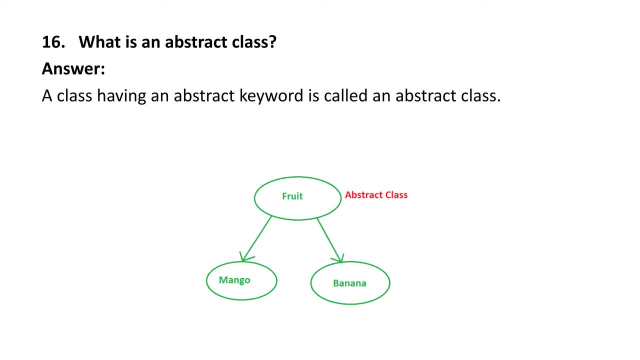 This can be understood with the help of this image. So here we have taken two classes: mango and bananas. So for these two fruits we have prepared a class that is fruit. So here fruit can act as an abstract class. Next question: what is an array? 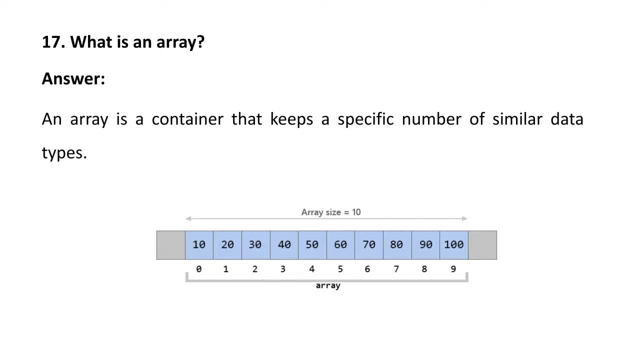 So the answer is: an array is a container that keeps a specific number of similar data types. So we can consider an array as a container where you can store a similar type of data, a homogeneous type of data. This can be understood with the help of this image. 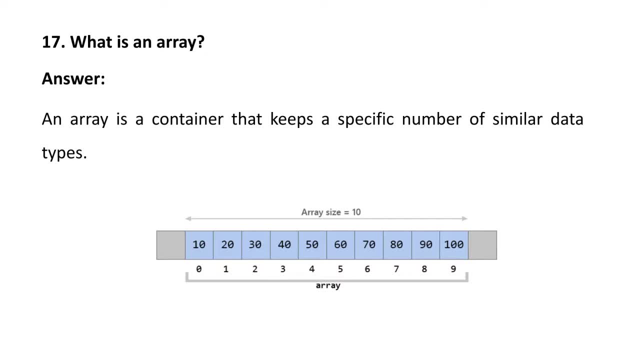 Here you can see one array. The size of this array is 10.. That means you can store 10 different values in this array. The condition is those values should be of same type. So here you can see. I have stored all the integers in that array. 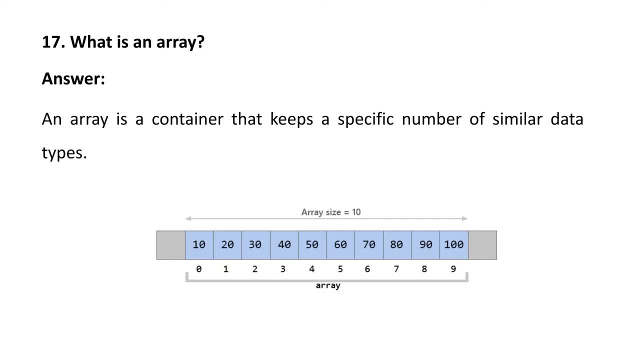 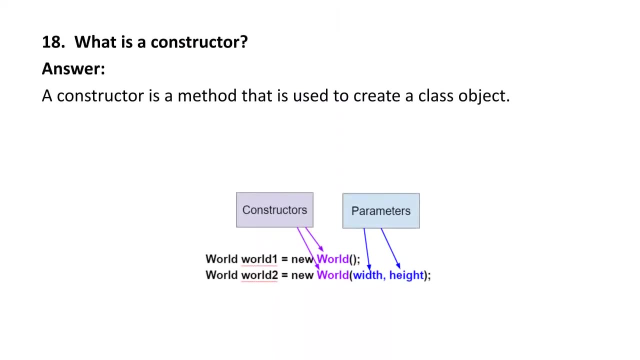 Then 0,, 1,, 2,, 3,, 4,, 5,, 6,, 7,, 8, 9.. This is nothing but the indices of that array. Next question: what is an array? The answer is constructor. 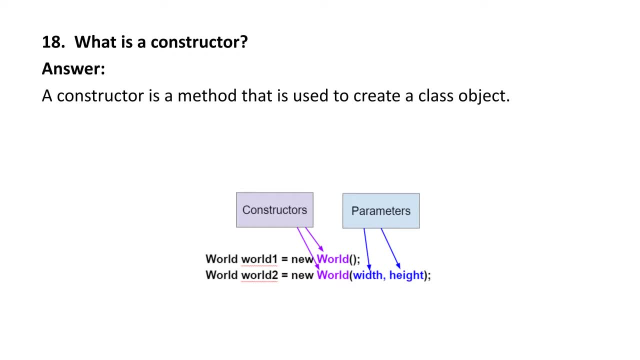 The answer is: a constructor is a method that is used to create a class object. So here you can see world. it is nothing but the constructor and its parameter is width and height. So the constructor is a method that is used to create a class object. 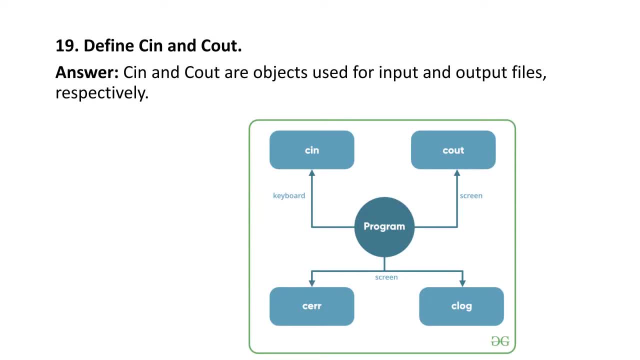 Next question: define cein and ceout. The answer is: cein and ceout are the object used for input and output files. So here you can see cein, that is, ceinput and ceoutput. So the input can be given with the help of keyboard and you can see the output over your screen. 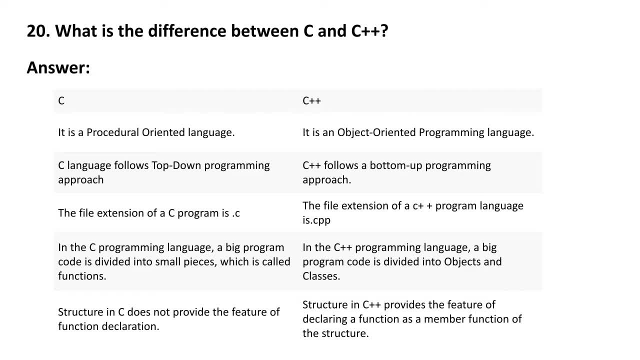 Next question: what is the difference between ce and ce++? This is the C language is a basic programming language. So we have two type of C languages. we can say that is ce and ce++. So the difference between ce and ce++: 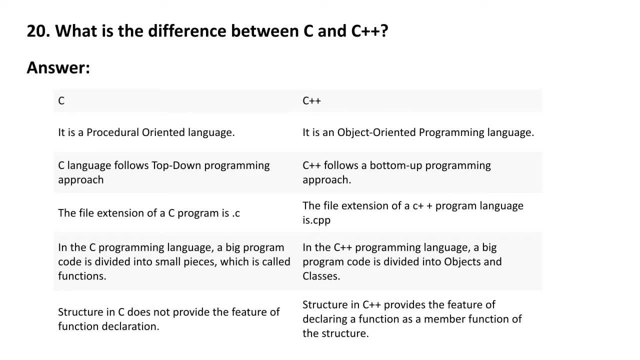 So the very first difference: ce is a procedure oriented language, Whereas ce++ is object oriented programming language. Then ce language follows top down programming approach, Whereas ce++ follows bottom up programming approach. Then the extension of ce program is cee, Whereas the extension of ce++ programming language. 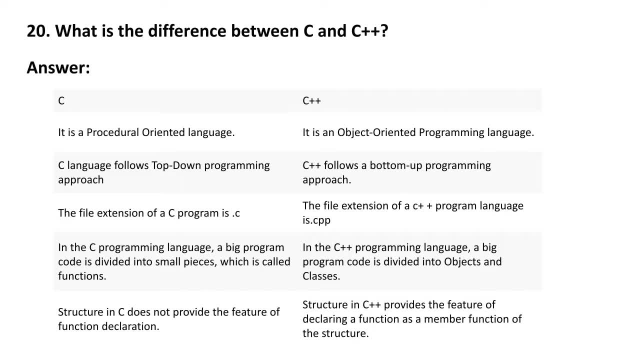 is cpp. Then in the C programming language a big program code is divided into small piece which is called as function. Then in the C++ programming language a big program code is divided into object and classes. Then structure in C does not provide the feature of function declaration. 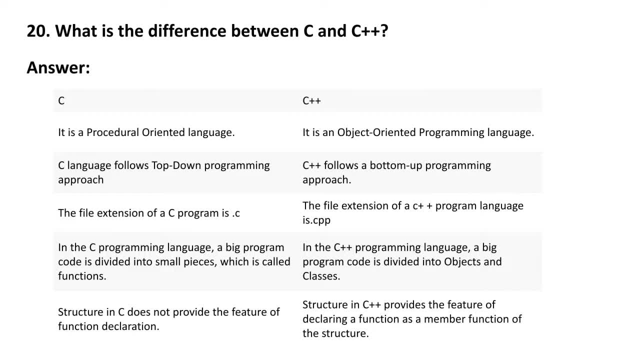 Whereas structure in C++ provide the feature of declaring function as a member function of the structure. So this is the difference between ce and ce++. So these are nothing but top 20 questions. technical interview questions. This video is useful for the fresher as well as experience candidate.